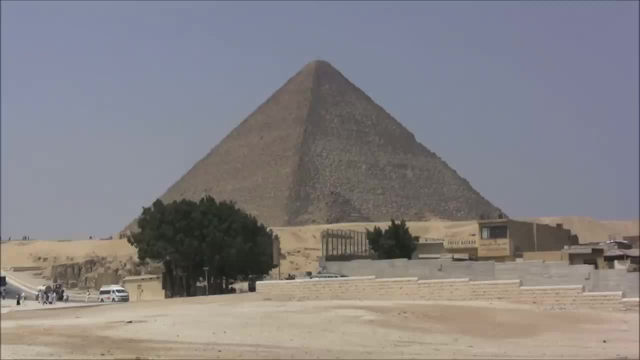 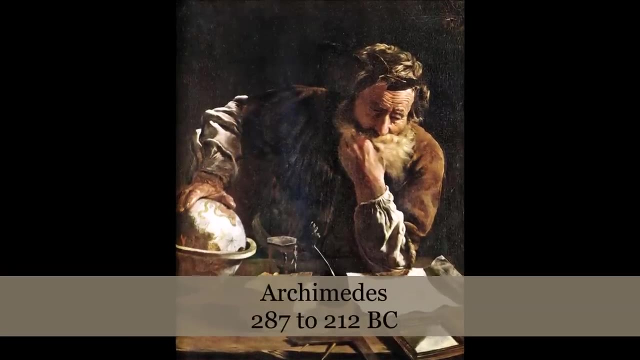 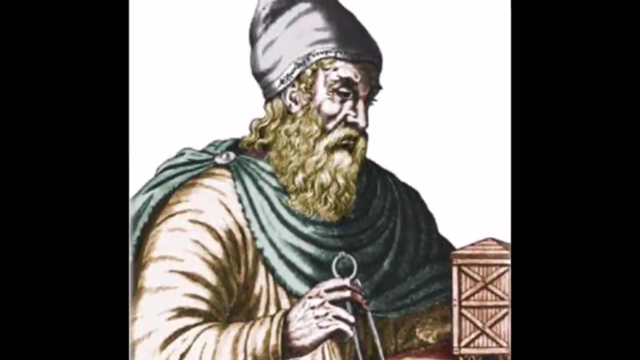 been known since prehistoric times and were used to help build the amazing structures left behind by ancient cultures. The Greek philosopher Archimedes identified three simple machines more than 2,000 years ago – the lever, the pulley and the screw He discovered. 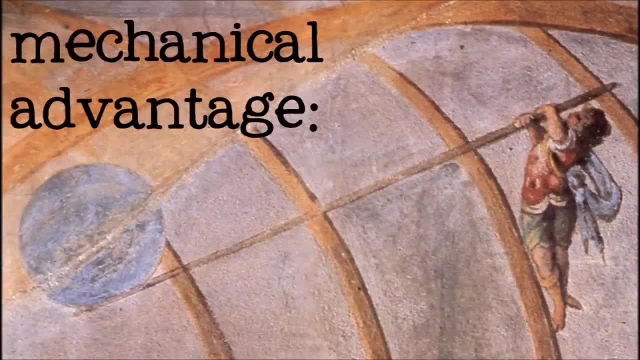 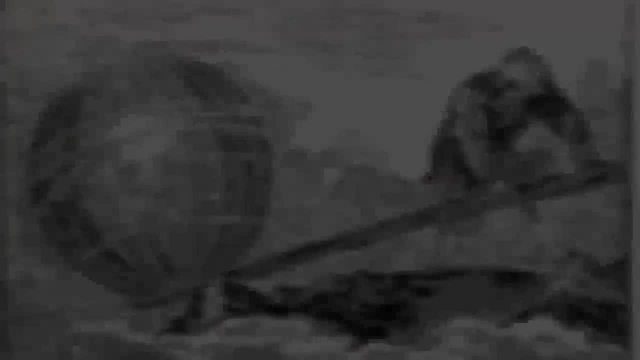 that a lever would create a mechanical advantage, which means that using a lever would allow a person to move something that would normally be too heavy for them to shift. Archimedes said that with a long enough lever and a place to rest it, a person could. 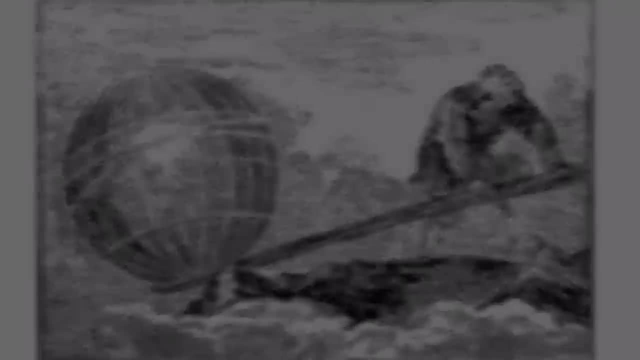 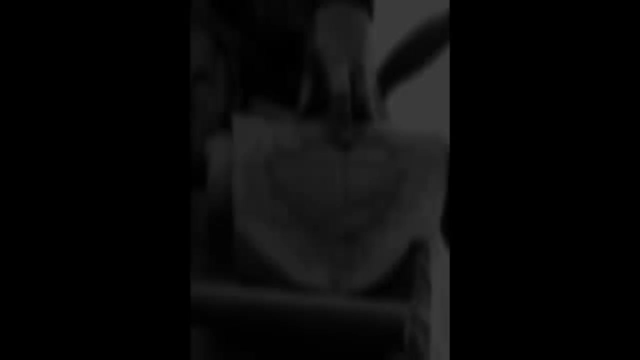 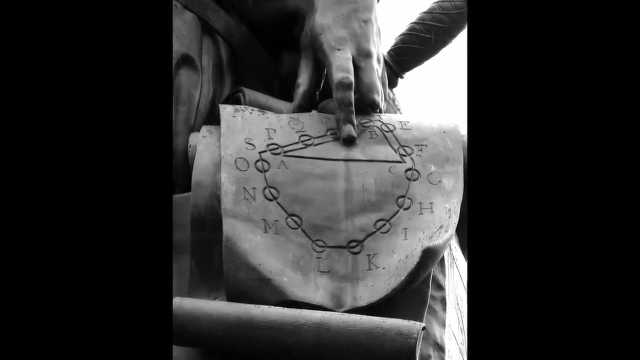 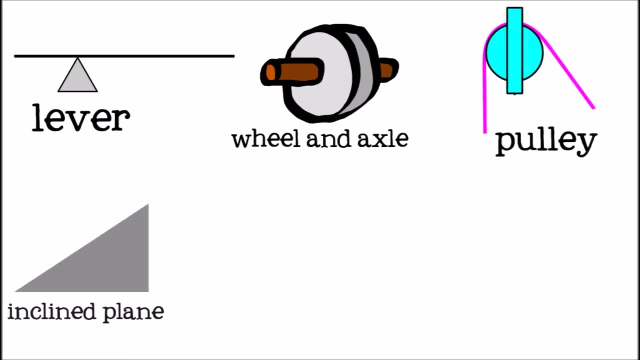 move the world Over the next few centuries. more simple machines were recognized, but it was less than 450 years ago that the last of the simple machines – the inclined plane – was identified. There are six types of simple machines – the lever, the wheel and axle. the pulley, the 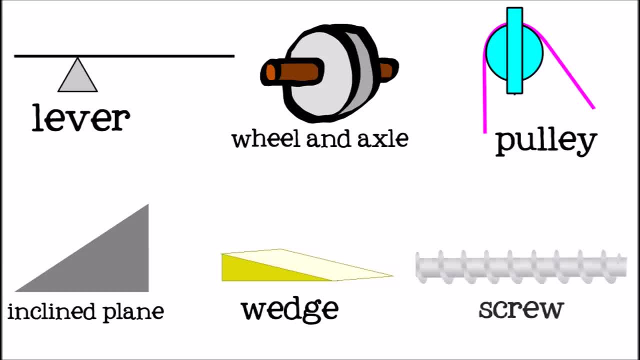 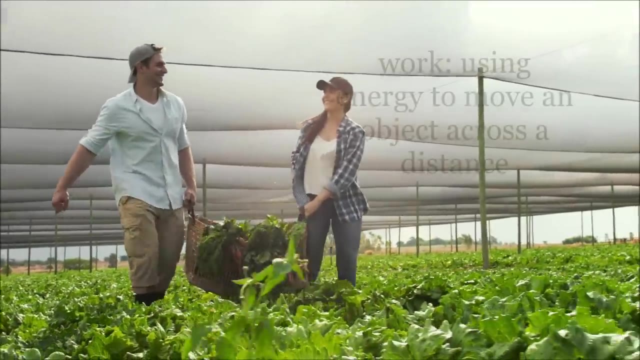 inclined plane. the wedge and the screw, Pulleys and wheel and axles are both a type of lever. Wedges and screws are both types of inclined planes. Each type of simple machine has a specific purpose and way they help do work. When speaking of simple machines, work means using energy to move an object across a distance. 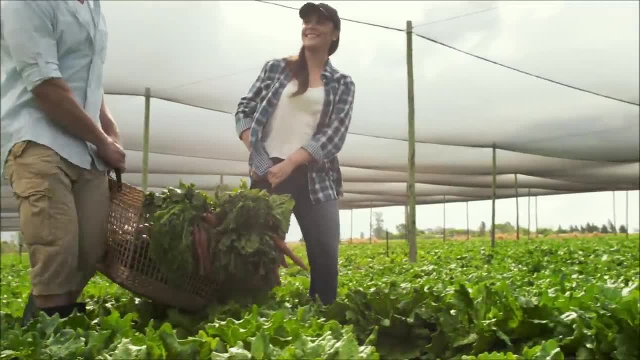 The further you have to move the object, the more energy you have to move the object- That's the most important thing about simple machines project- the more energy it takes to move it. Let's see how each type of simple machine helps do work. 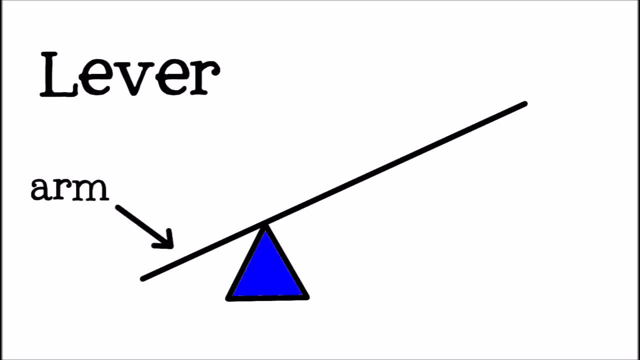 A lever is a tool like a bar or rod that sits and turns on a fixed support called a fulcrum. When you use a lever, you apply a small force over a long distance and the lever converts it to a larger force over a shorter distance. Some examples of levers are seesaws, crowbars. 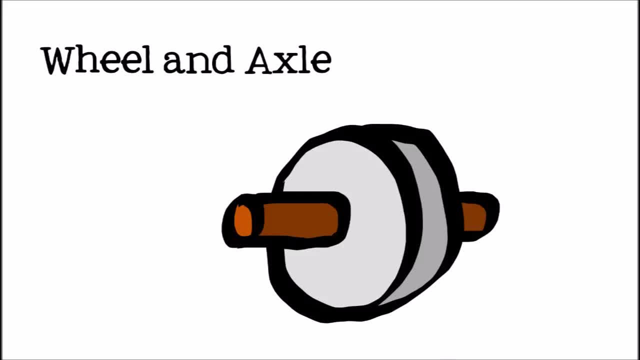 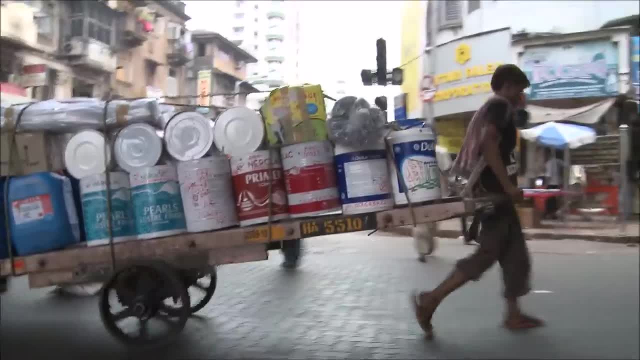 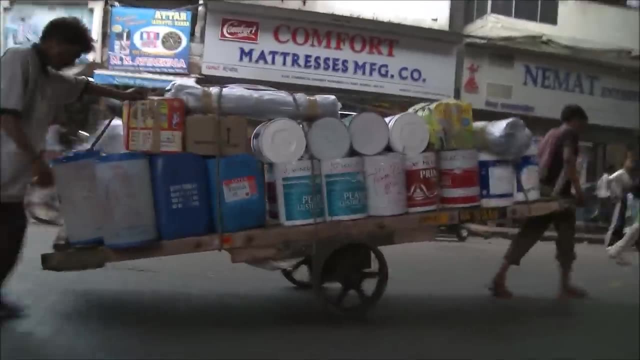 and tweezers. A wheel and axle is easy to recognize. It consists of a wheel with a rod in the middle. You probably already know that it's easier to move something heavy if you can put it in something with wheels, but you might not know why. 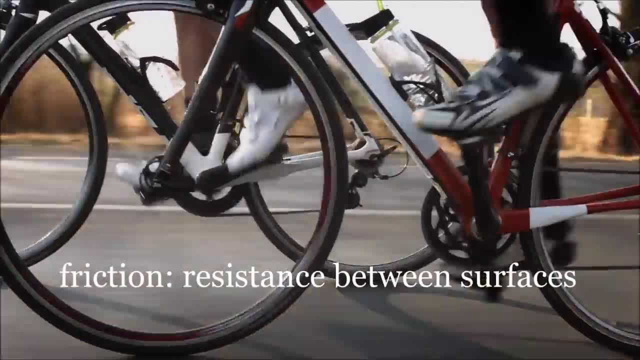 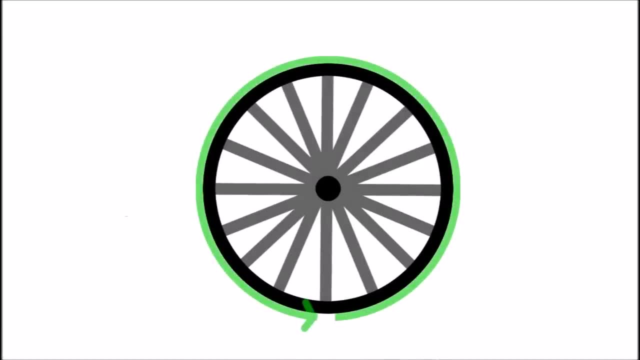 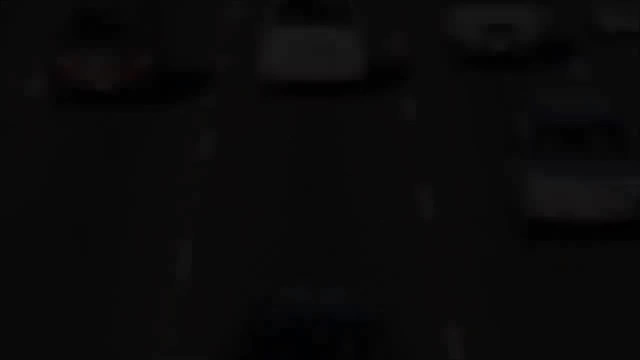 For one thing, using wheels reduces the friction or resistance between surfaces, between the load and the ground. Secondly, much like the lever, a smaller force applied to the rim of the wheel is converted to a larger force traveling a smaller distance at the axle. 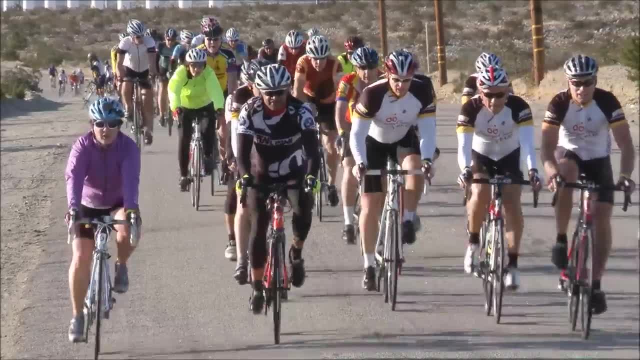 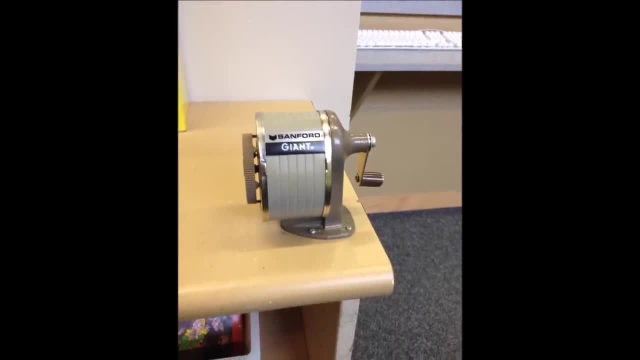 Wheel and axles are used for machines such as cars, bicycles and scooters, but they are also used in other ways, like doorknobs and pencil sharpeners. A pulley is a machine that uses a wheel with a rope wrapped around it. The wheel often 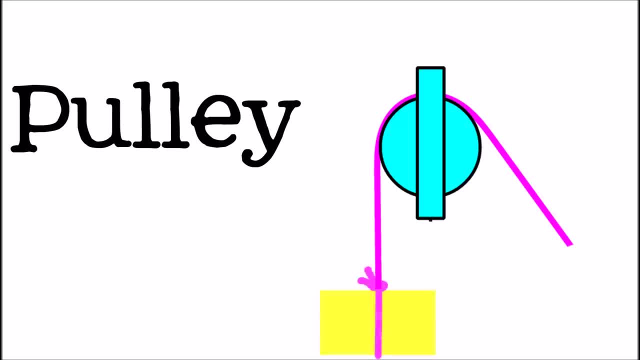 has a groove in it which the rope fits into. One end of the rope goes around the load and the other end is where you apply the force. Pulleys can be used to move loads or change the direction of the force you are using and help make work easier by allowing you. 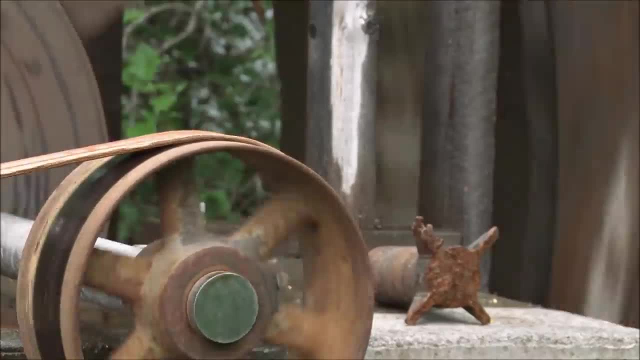 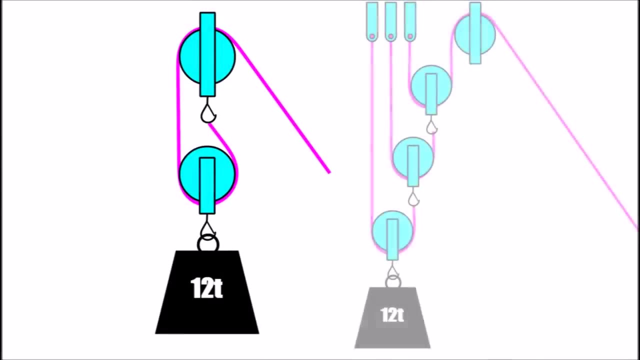 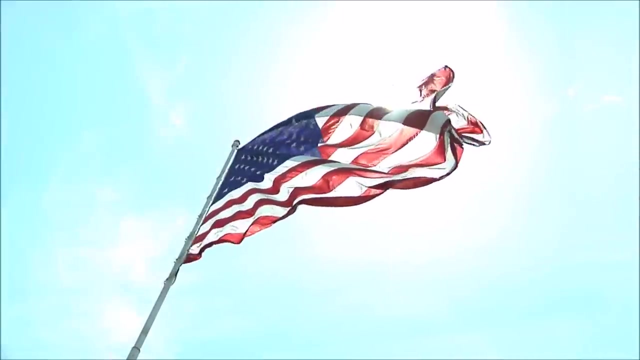 to spread a weaker force out along a longer path to accomplish a job. By linking multiple pulleys together, you can do the same job with even less force, because you are applying the force along a much longer distance. Pulleys may be used to raise and. 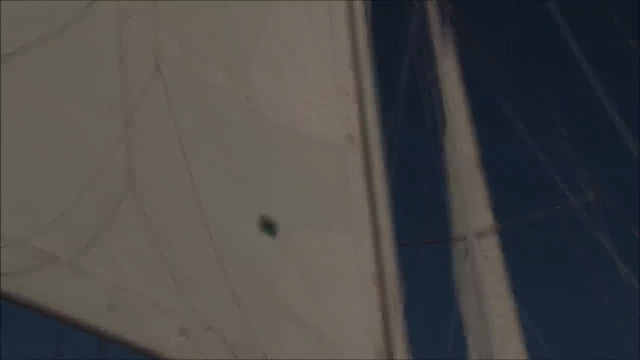 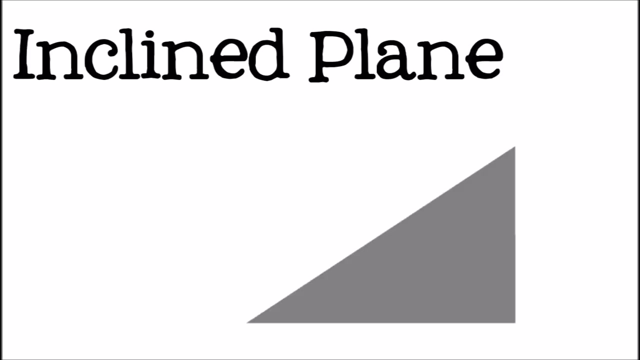 lower flags, blinds or sails and are used to help raise and lower elevators. An inclined plane is a flat surface with one end higher than the other. Inclined planes allow loads to slide up to a higher level instead of being lifted, which allows the 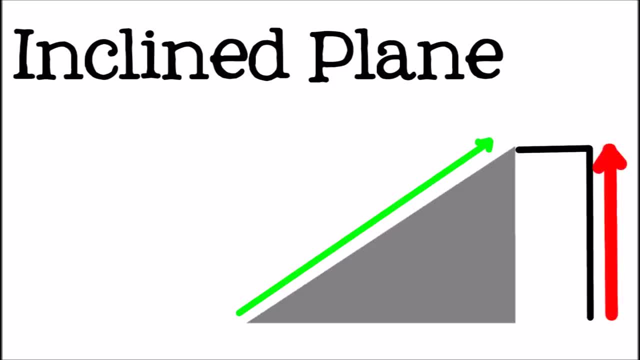 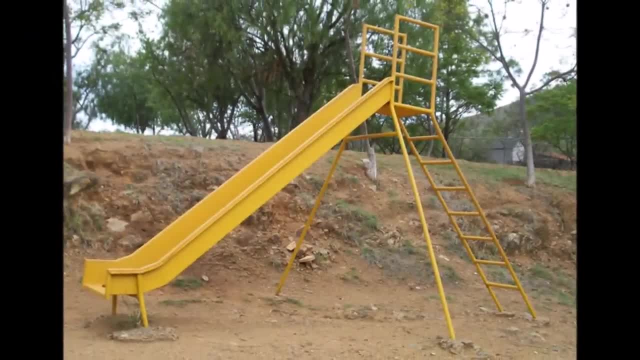 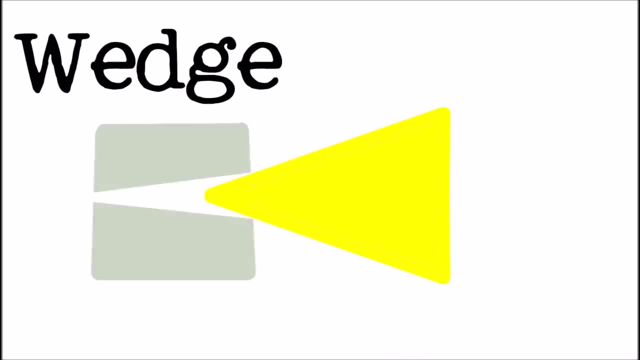 work to be accomplished with a smaller force spread over a longer distance. You may recognize an inclined plane as the simple machine used in ramps and slides. A wedge is simply two inclined planes placed back to back. It is used to push two objects apart. A smaller force applied to the back of the wedge is converted to a greater force. 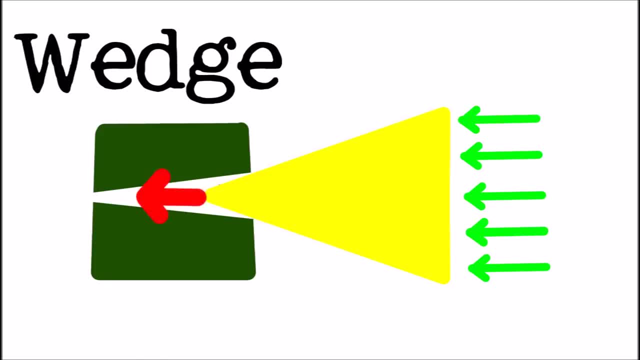 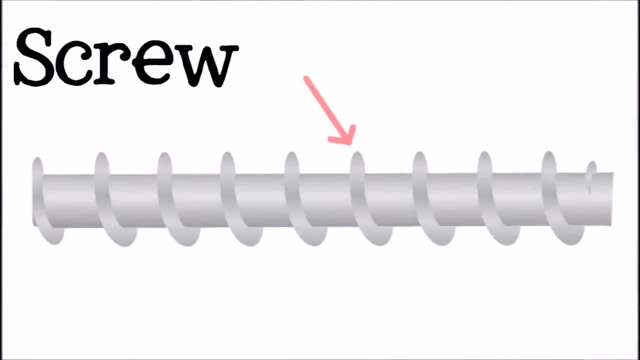 in a small area at the tip of the wedge. Examples of wedges are axes, knives and chisels. A screw is basically an inclined plane wrapped around a pole. Screws can be used to hold things together or to hang a board. 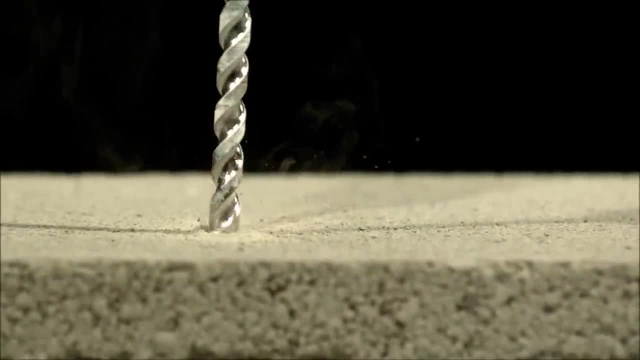 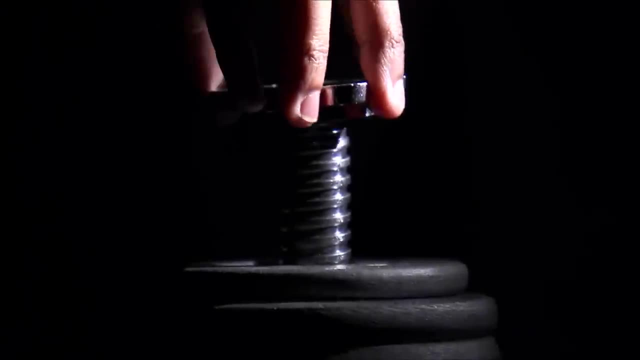 or to hold a lighter, lift things Just like the inclined plane. the longer the path the force takes, the less force is required to do the work. Screws with more threads take less force to do a job, since the force has to travel a longer distance.